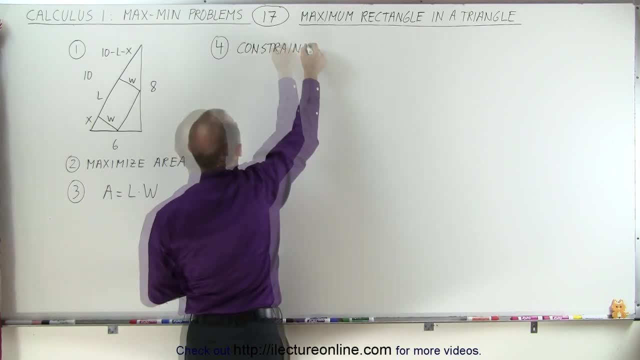 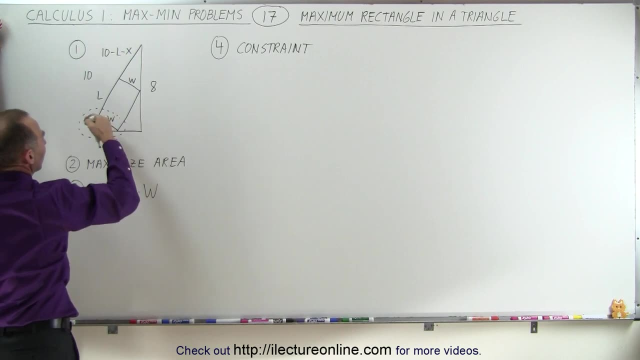 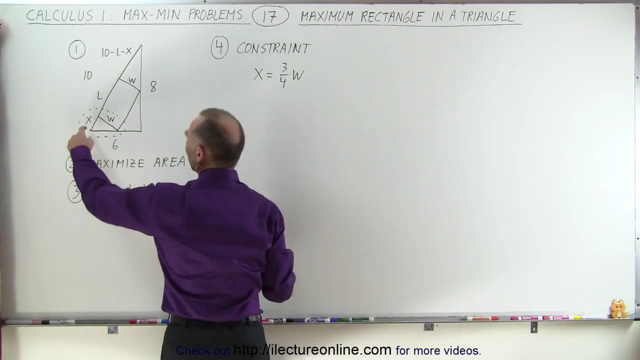 trying to find the constraint. Well, first of all, let's take a look at the triangle right here. We know because of similarities that this also needs to be a three, four, five triangle, which means the relationship here between x and w can be expressed as: x is going to be equal to three quarters w, because this has to be a three- four. 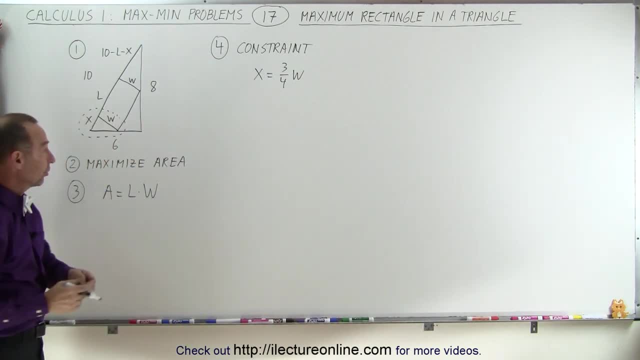 five triangle as well, At least the ratio same as the ratio of the big triangle. All right, now we have w. now we have to find the ratio of the big triangle. So we're going to take a look at this and we're going to have to somehow convert that to l right. We need to relate w and l, which means we 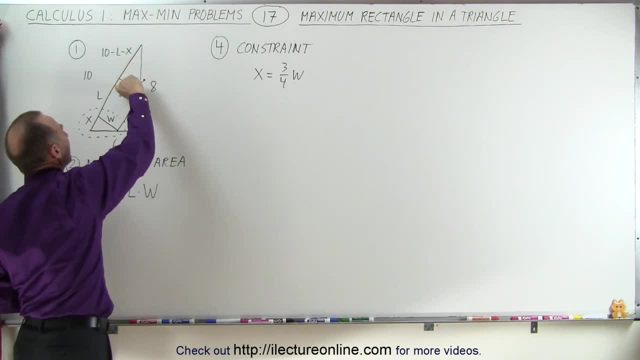 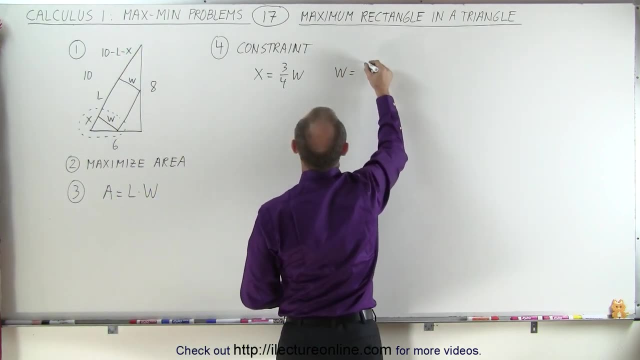 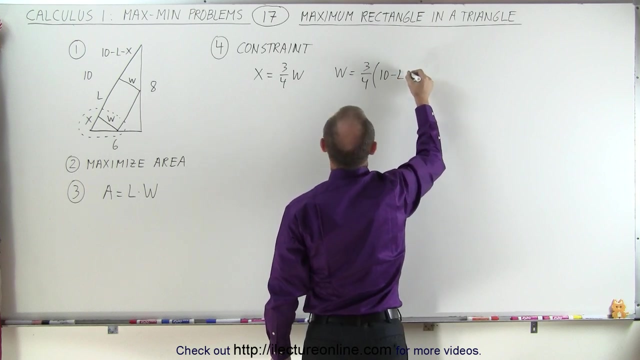 can go to this triangle right here and do the same thing. We can say that w is equal to three quarters this distance. So let's try that W is equal to three quarters this distance right here, which is ten minus l minus x. Remember, we're trying to relate x, we're 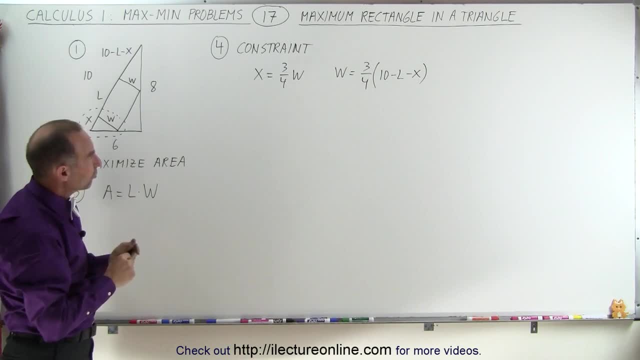 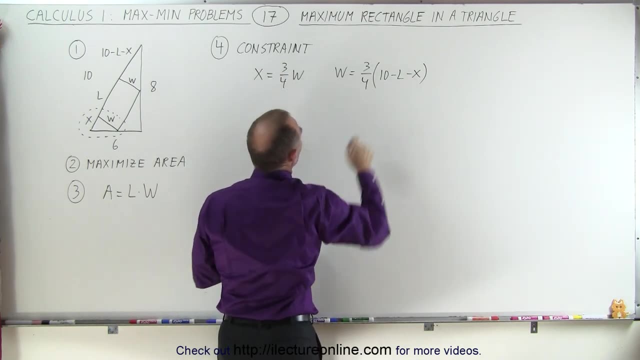 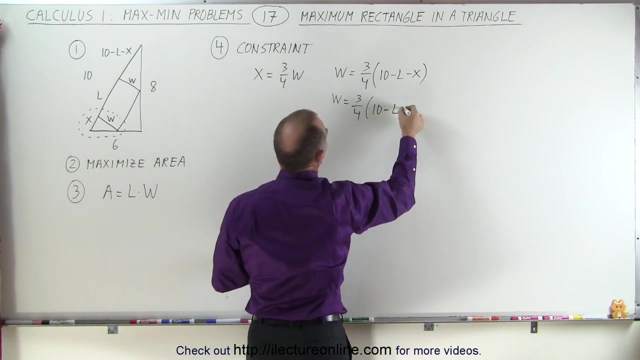 W to L, so we can limit one of the variables, which means we need to get rid of an X here, and since X could be written as 3 quarters W, that can go in here. so W is equal to 3 quarters times 10 minus L minus X, which is 3 quarters W. 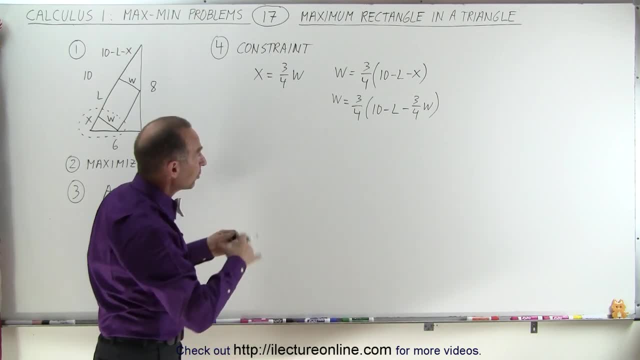 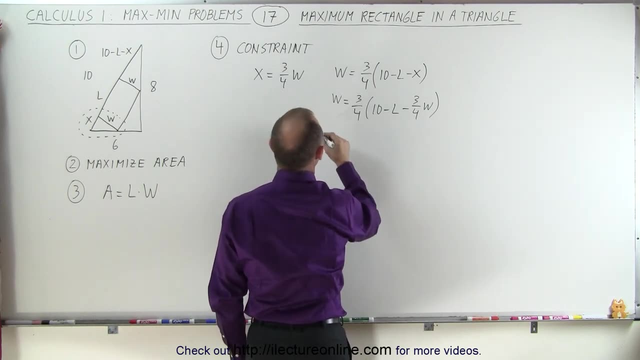 now I think we're ready to relate L to W. we just need to do a little algebra. so let's go ahead and multiply this out, or maybe what I need to do here is move this to the other side. let's do that so we have 4 thirds. W is equal to 10 minus. 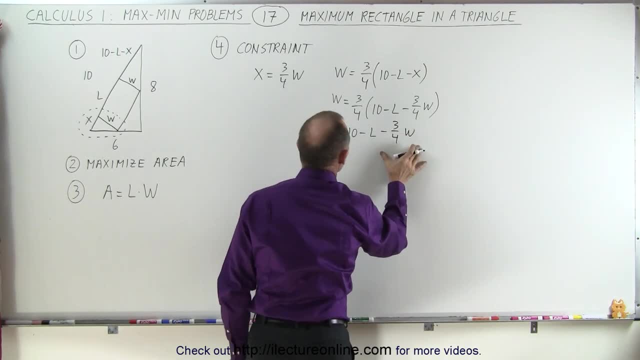 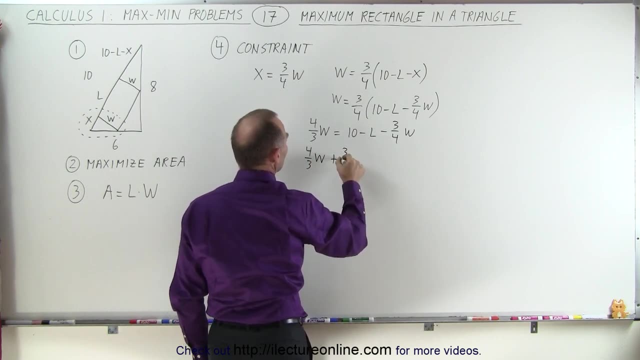 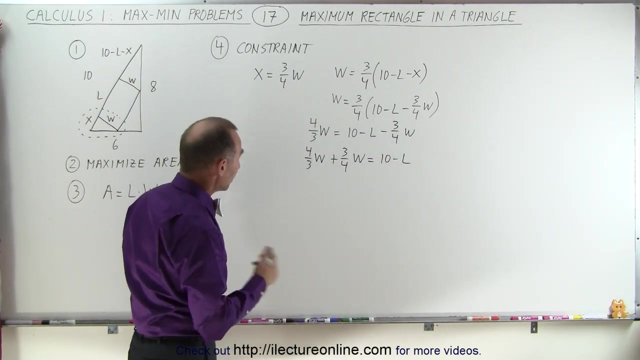 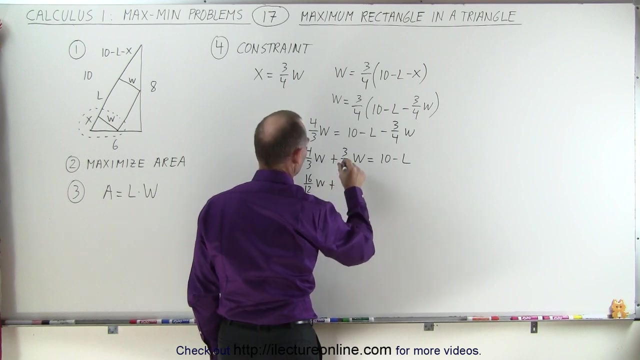 L minus 3 quarters W. so move all the W's over to one side. we have 4 thirds W plus 3 quarters W is equal to 10 minus L. now I need a common denominator, which would be 12, so let's do that. so 3 goes in 12 four times, that's 16 over 12 W plus that goes in 12 three. 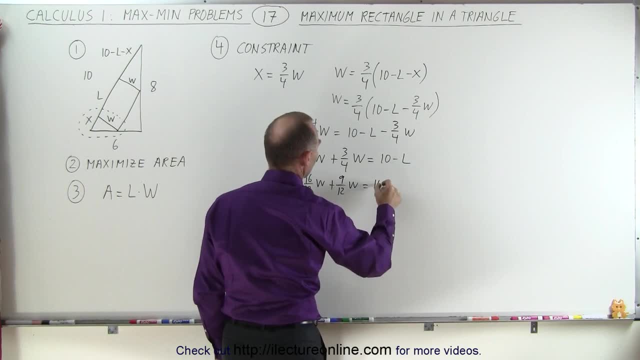 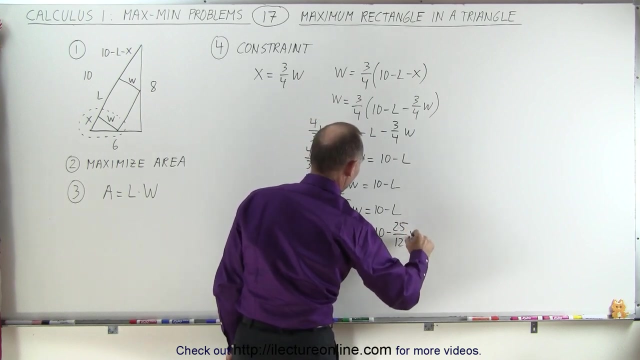 times or 9 over 12 W equals 10 minus L. together, that is 25 over 12 W equals 10 minus L, or L is equal to 10 minus 25 over 12 W, and that can go into my original equation where express area: 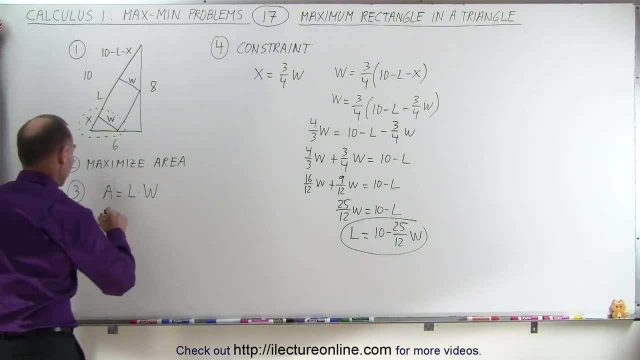 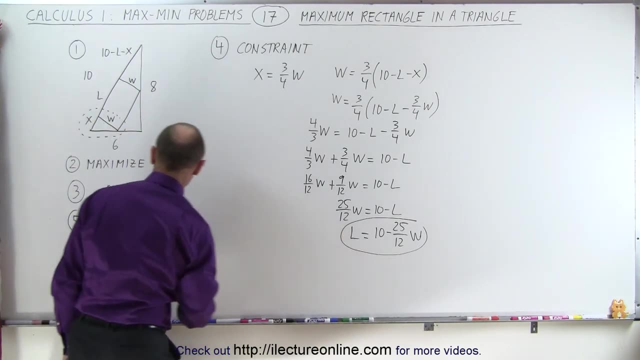 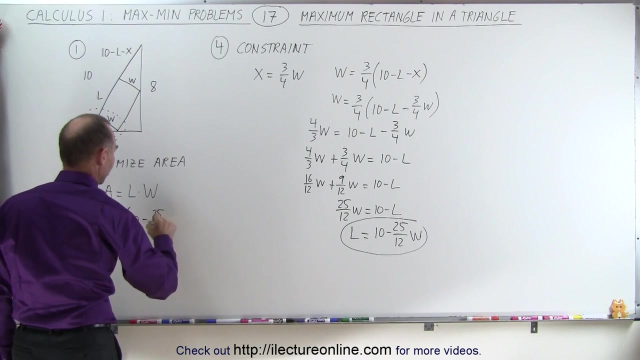 in terms of L and W and that way get rid of L. so now we have. so that would be step 4. step 5 would be to substitute for L what L is equal to. so we have a is equal to the quantity 10 minus 25 over 12 W times W, and simplifying this, we get. 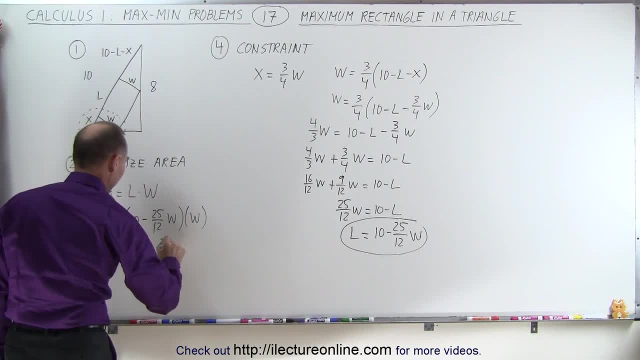 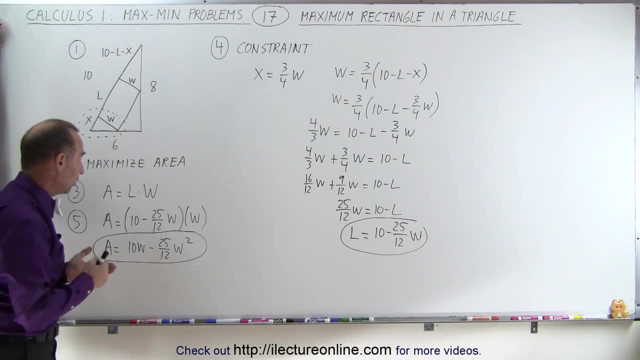 a is equal to 10 W minus 25 over 12 W squared. so now we have a equation where we have the area which we're trying to maximize in terms of W alone. now we can go to the next step, where we take the derivative and set the. 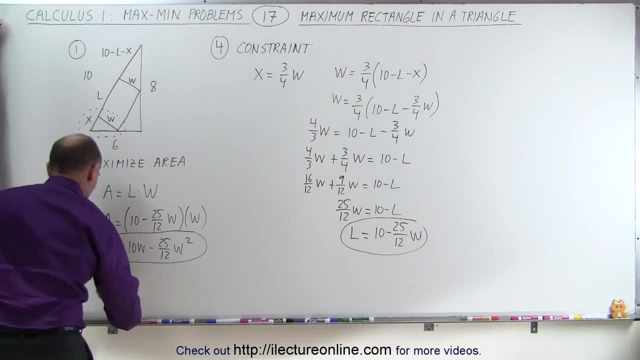 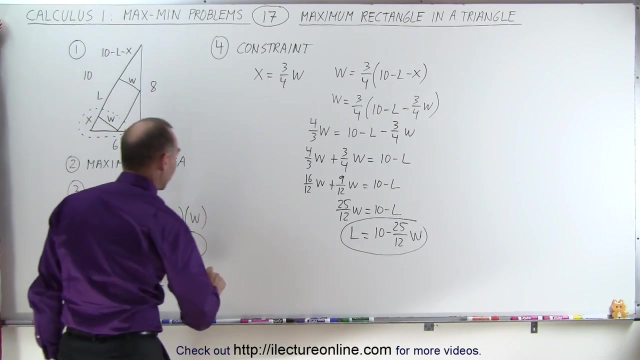 derivative equal to 0, so a prime- it's going to be 10 minus 2 times 25 is 50 divided by 12 can be written as 25 divided by 6, so 25 divided by 6, W. and then we're going to set: and oh, I'm running out of room here, so let's go. 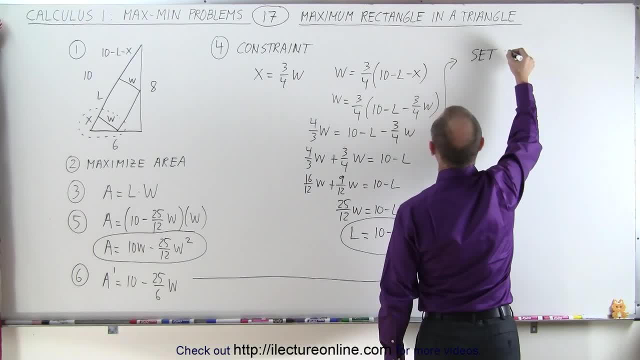 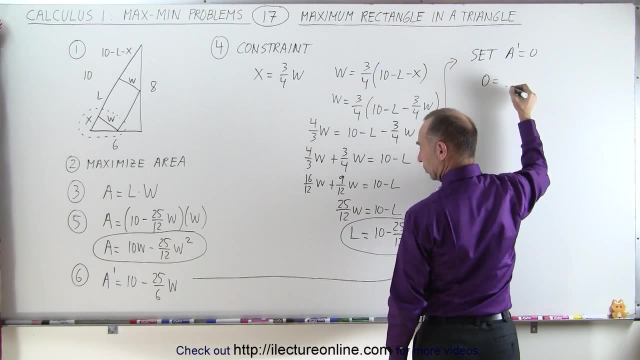 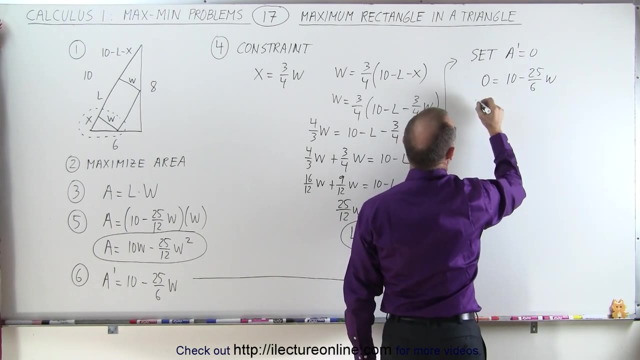 over here. now we're going to set the area prime equal to 0, so we can solve for W. so we get: 0 is equal to 10 minus 25 over 6 W. moving this to the other side, I can say that 25 over 6 W equals 10, or W is equal to 60 divided by 25. 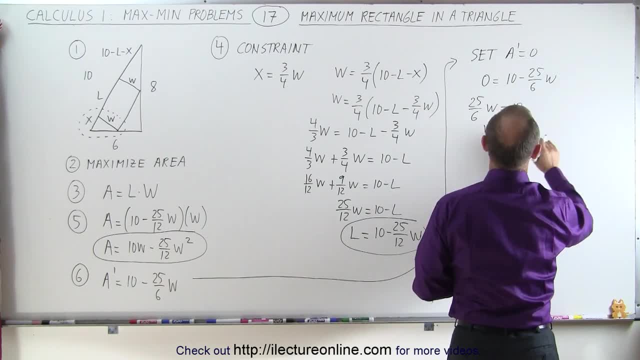 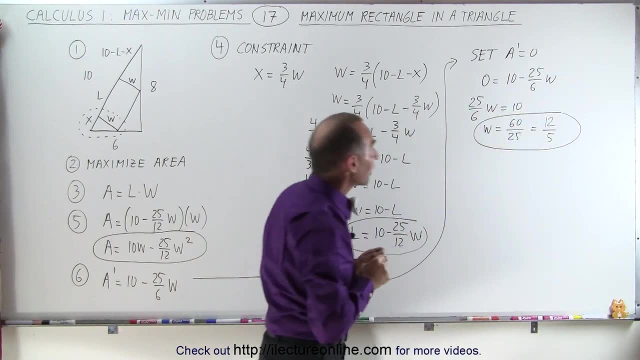 can reduce that to divide both top and bottom by five. we have 12 divided by five. so there's the value of the width of the rectangle, 12 divided by 5.. now when we plug that into the equation over here, we can solve for the length of the rectangle. so we get length is equal to 10 minus 25 over 12.